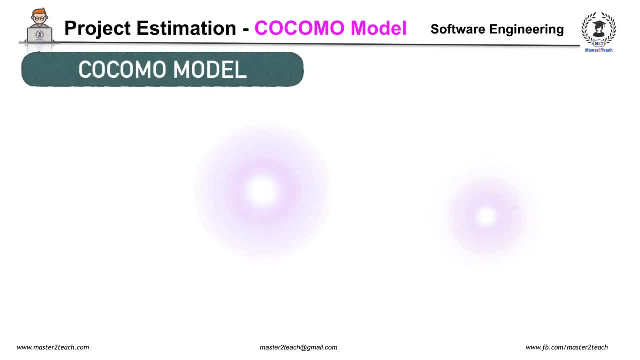 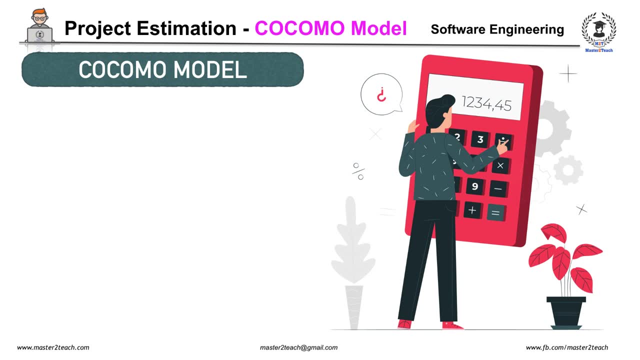 which we are going to learn in this tutorial. Kokomo models. Cost of the project is one of the most challenging job for the software engineer. One of the best way to calculate the cost of the project is COCOMO. COCOMO stands for constructive cost model. 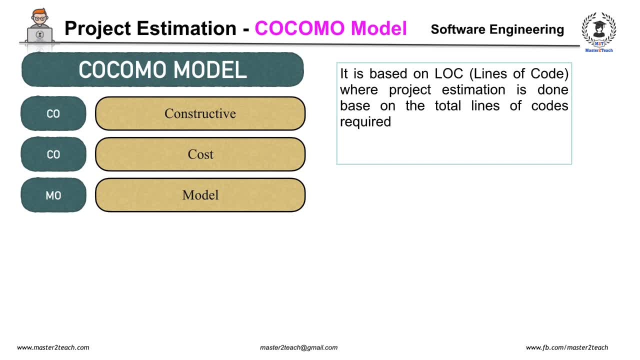 It is based on lines of code, where project estimation is done based on the total lines of codes required to develop the system. That is. size of the system defines the cost of the project. COCOMO was first developed by Barry Boehm in 1981 as a model that is used to estimate. 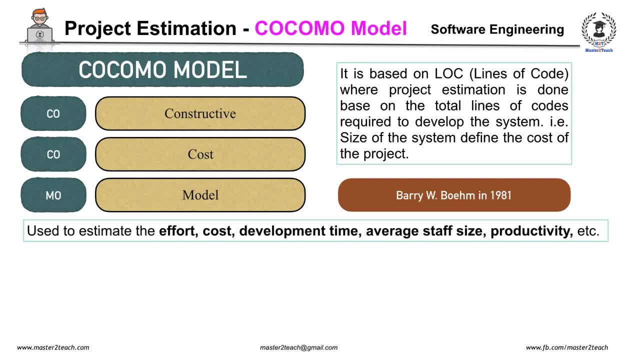 the effort, cost, development, time, average staff size, productivity, etc. It is a hierarchy of software cost estimation models. It consists of three hierarchies increasingly detailed and accurate forms: Number one: basic- COCOMO model. Number two: intermediate- COCOMO model. 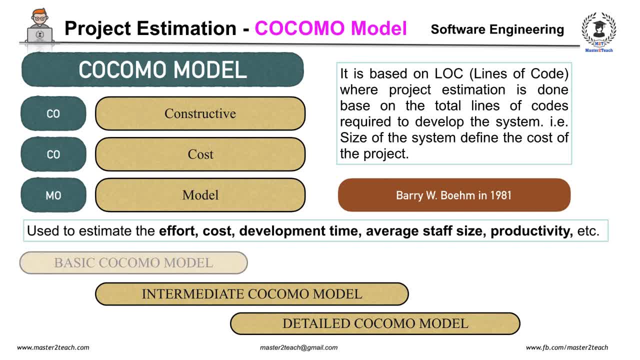 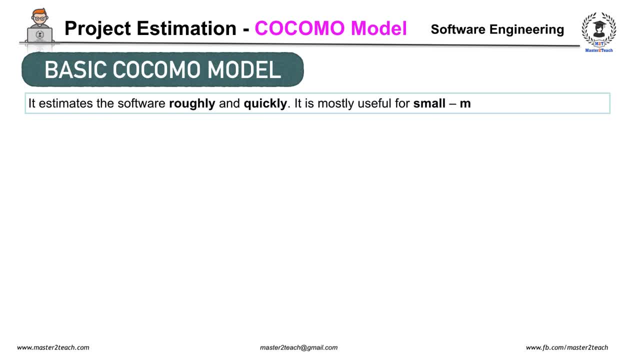 Number three: detailed COCOMO model. We will learn basic COCOMO model. Basic COCOMO model. It estimates the software roughly and quickly. It is mostly useful for small to medium-sized software. There are three modes of development: organic, semi-detached and embedded. 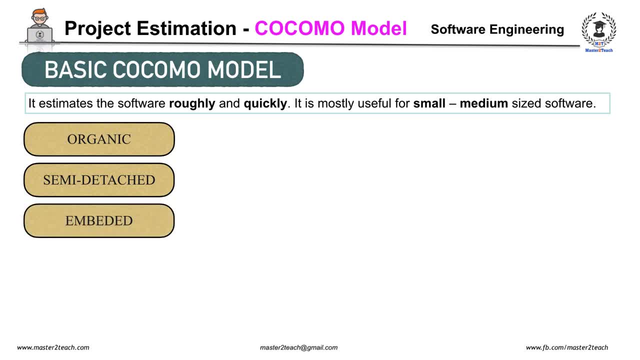 We use these three different modes of development to calculate the project effort, development time, average staff size, productivity, according to different criteria which are as follows. Basic model equation: Effort is equal to A Multiplication of thousands lines of code. KLOC to the power B, which units is person. 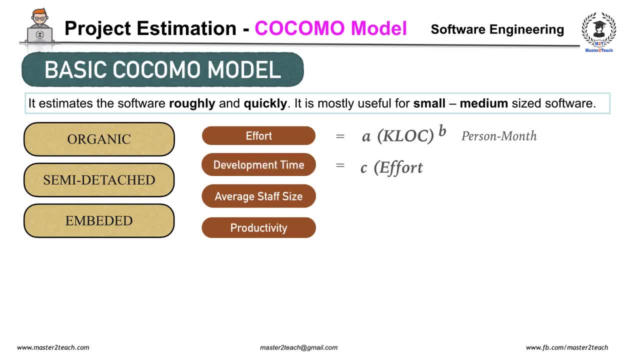 months. Development time is equal to C Multiplication effort to the power D, which units is months. Average staff size is equal to effort divided by development time, which units is persons. Productivity is equal to KLOC divided by effort, Where A, B, C and D are the constants whose values for different modes of development. 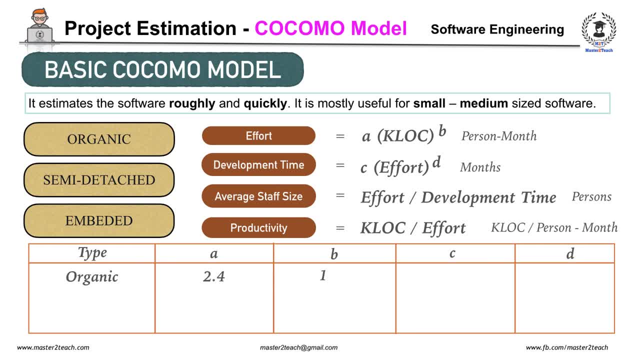 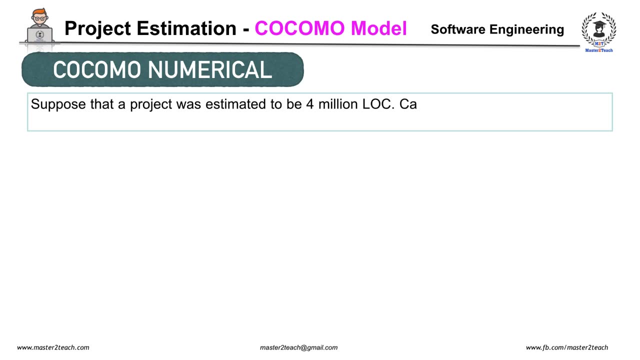 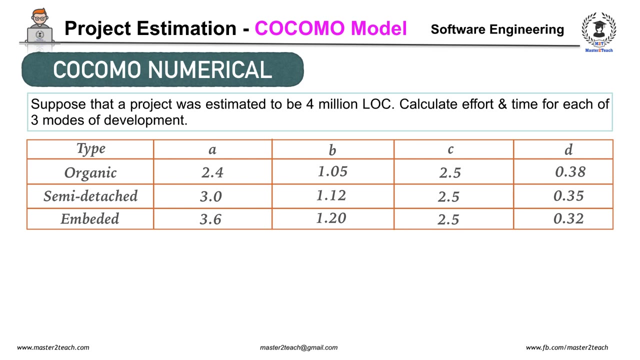 are as follow. Now let's go through the example of the COCOMO model numerical equation. Suppose that a project was estimated to be four millions lines of code. Calculate the initial number of lines of code. KLOC, effort and time for each of three modes of development.